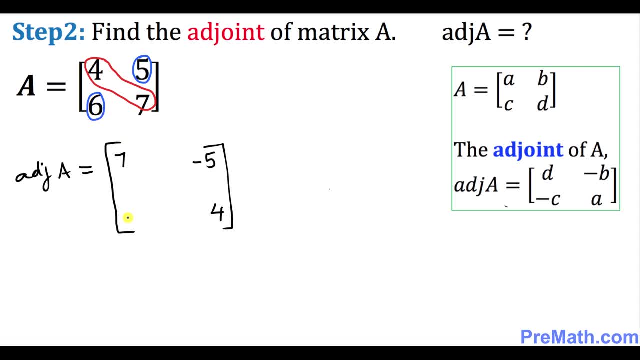 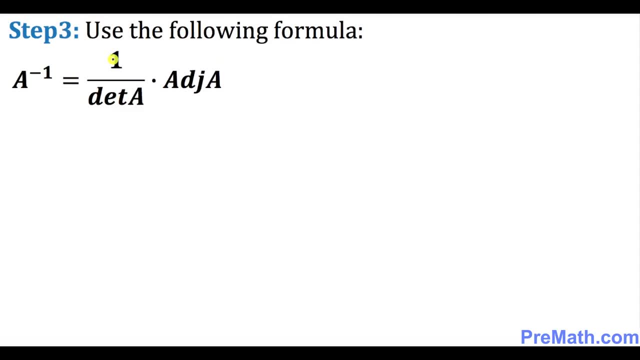 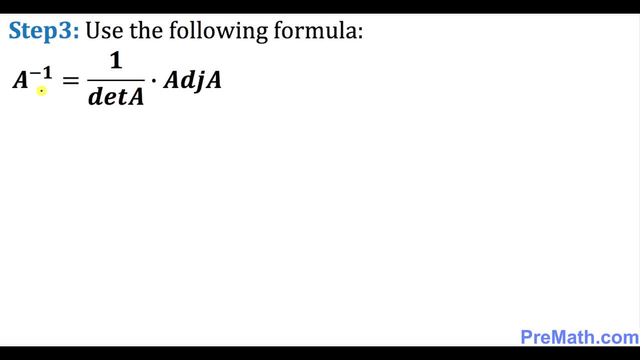 using this formula to find the inverse matrix A. So 1 over determinant of A times ADJ of A. and here are these values: determinant of A is negative 2 and this is ADJ of A that we found out in our previous steps. Let's go ahead and apply those values in this formula. So A inverse. 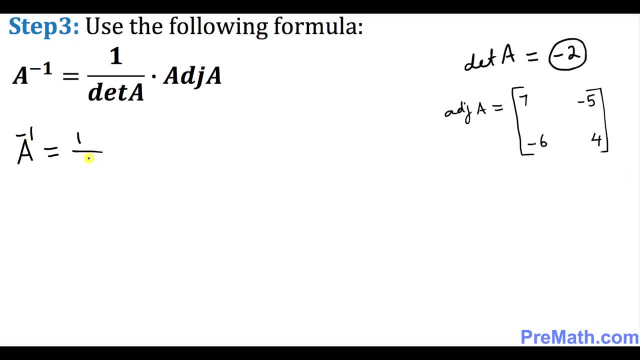 turns out to be equal to 1 over negative 2 times. go ahead and put down our adjoint matrix, which is 7 negative, 5 negative, 6 and 4.. Now, since this fraction 1 over negative 2 is multiplying with this matrix, so that means this fraction is going to get multiplied with each and 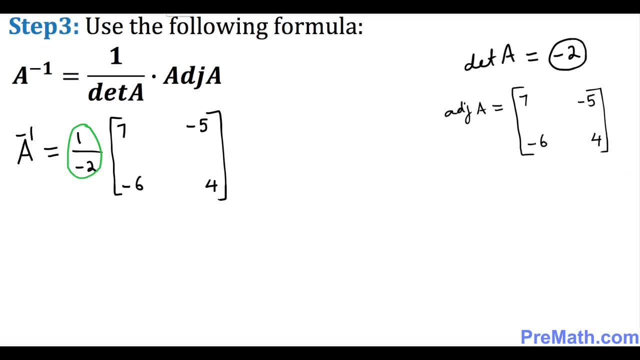 every element of this matrix. So let's go ahead and multiply it out, so that's going to be simply 7 over negative, 2, negative 5 over negative 2, negative 6 over negative 2 and 4 over negative 2.. Let's reduce these fractions and simplify them, so that is going to turns out to be negative 7. 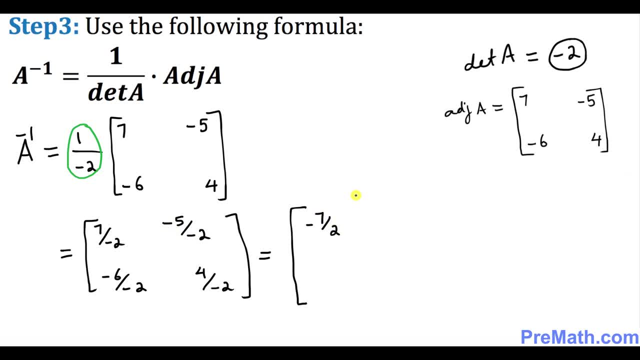 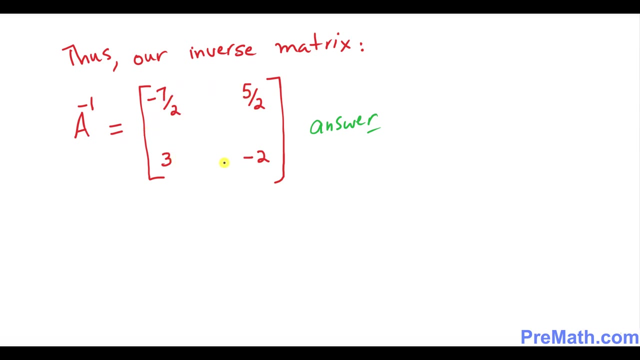 over 2.. This negative and negative become positive, so that's going to be 5 over 2.. These again, this fraction turns out to be 3, and that's going to be negative: 2, and that is our inverse matrix. Thus, our inverse matrix turns out to be this: 1, as you can see, and that is our answer. Thanks, 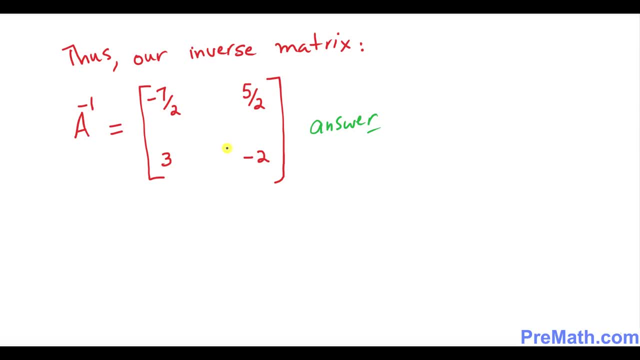 for watching and please subscribe to my channel For more exciting videos.